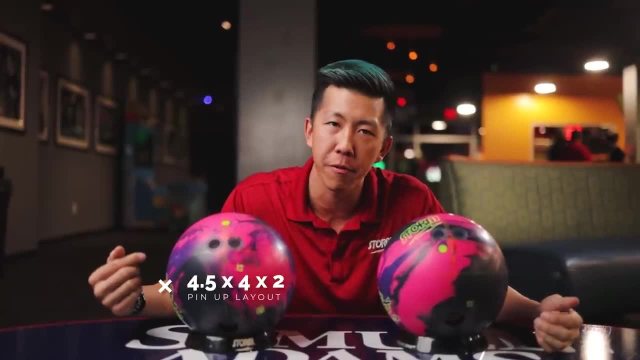 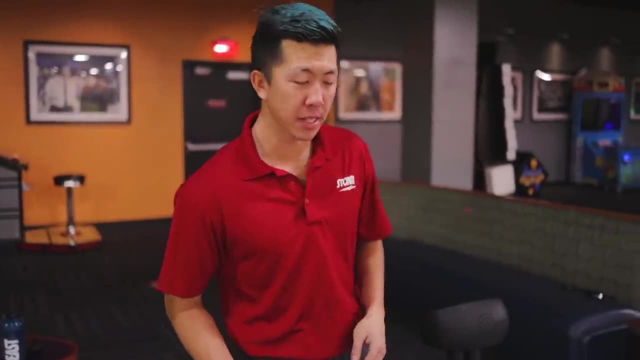 And this is for asymmetric bowling balls. This is going to be a 4.5x4x2 layout for the pin up layout and the pin down is going to be a 5x5x4.5.. So we got our pin up and pin down Proton PhysX here. 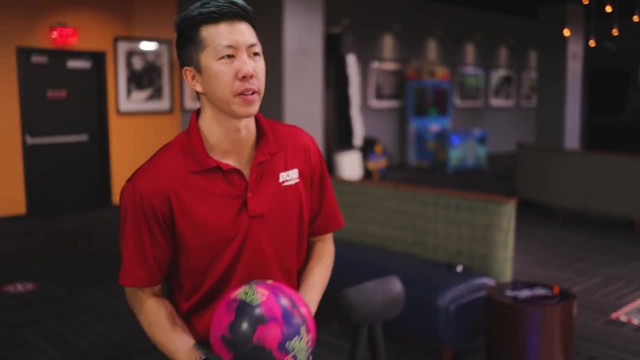 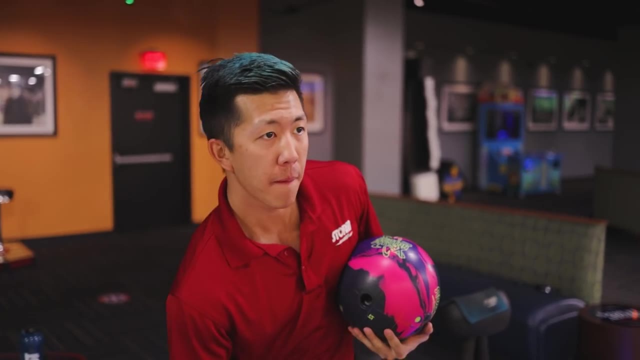 I'm going to start with the pin down one, because it allows me to play a little straighter, And we'll talk a little bit about pin up versus pin down layouts in general a little later. First, we're going to test out these bowling balls and see how they look. 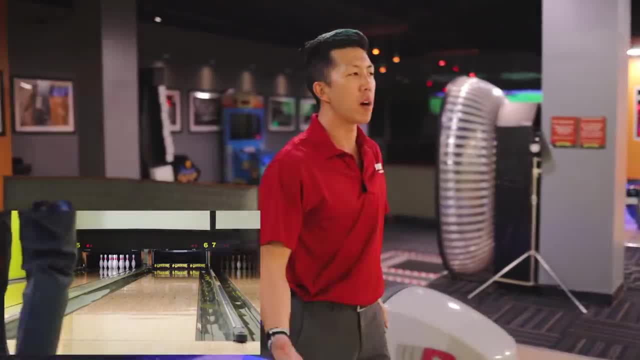 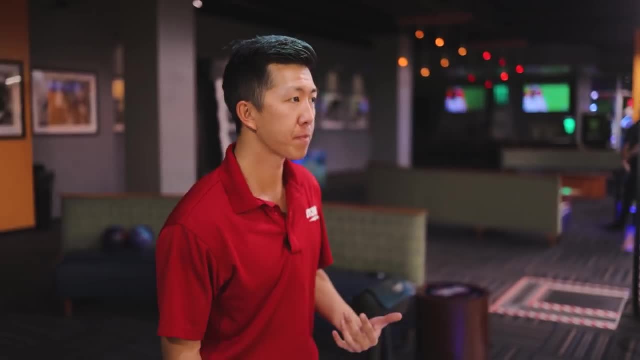 All right. so we got the pin down ball right there and what I'm expecting: the different layouts. the pin down one should be a little bit longer and a little smoother because of the flare, And the pin up one is probably going to force me much further left. 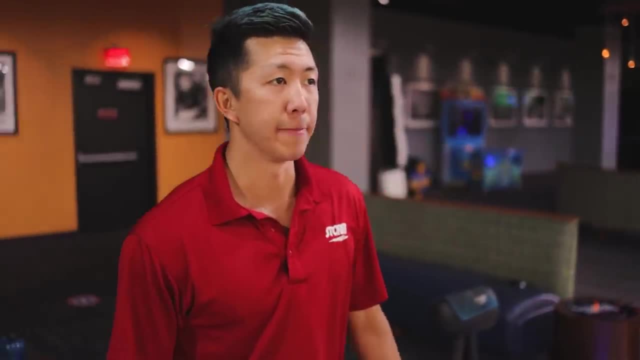 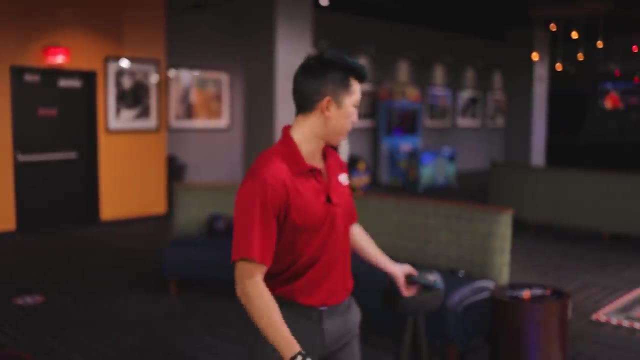 It's going to want to flare a lot more and probably hook earlier as well. And yeah, we'll give the pin down one another. look, I'm thinking we're just going to drop the speed a touch just to get it to pick up a little sooner. 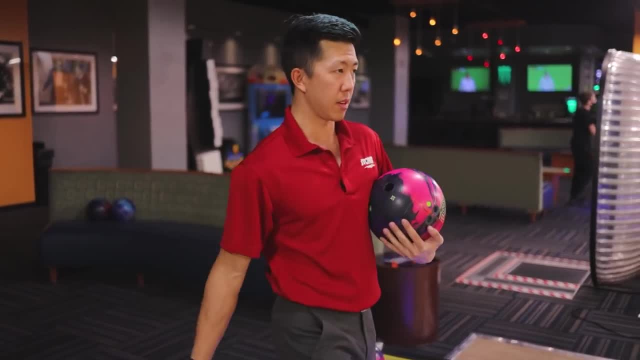 I'm not going to move my foot, I'm just going to try to get it to pick up a little sooner. I'm not going to move my foot, I'm just going to try to get it to pick up a little sooner. Keep things the same. 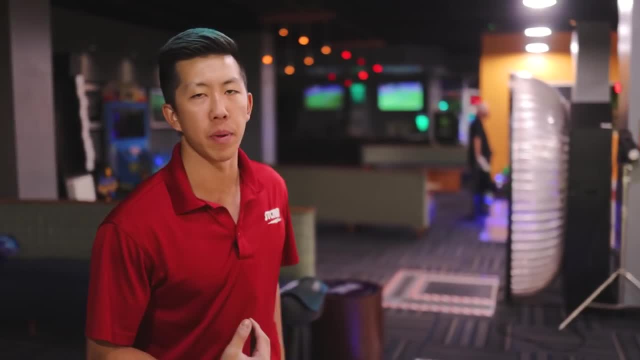 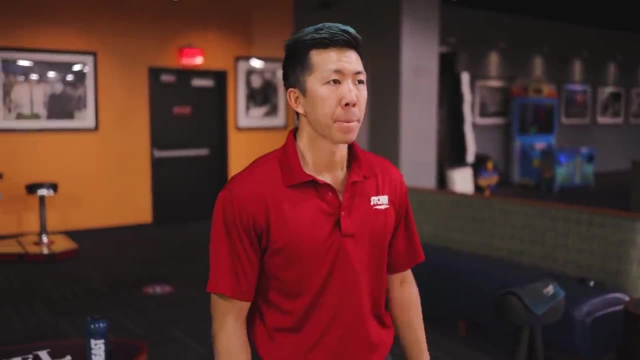 So you kind of see the ball really wants to stay on line. I went a notch lower with my ball speed still kicking the 10, not quite flush yet. so I could probably afford to move a little further right with my feet. But I'm not going to do that and I'm just going to try the pin up ball. 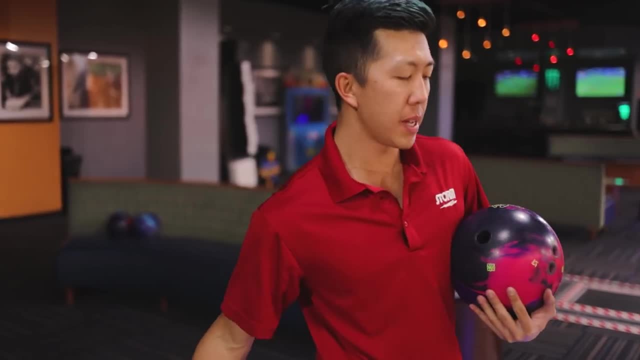 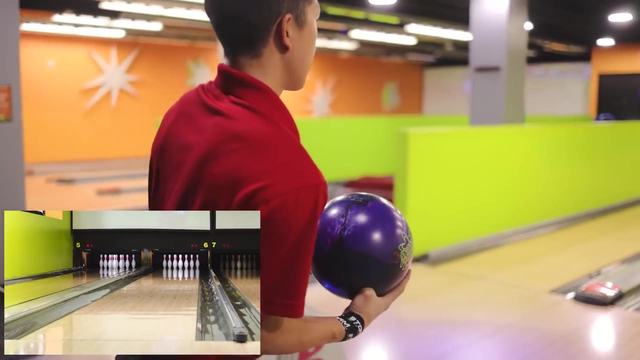 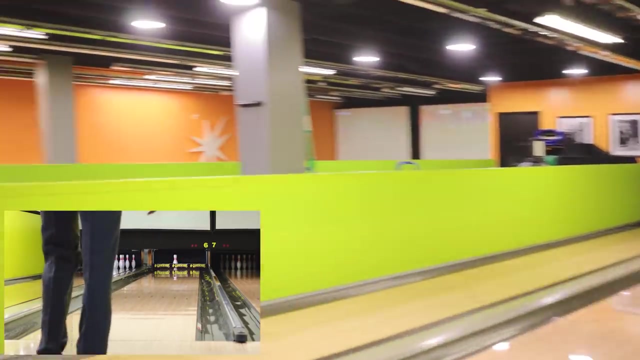 Okay, so here we got our pin up ball and a half inches from our PAP. I'm going to stay in the same spot and we'll see what this one gives us. That wasn't my best shot. Then I went into the ground, So I'm going to make the same adjustment. 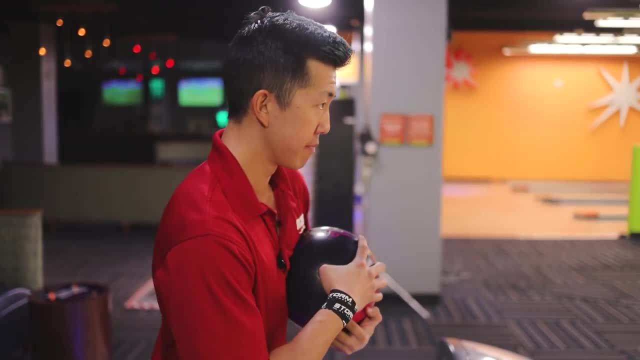 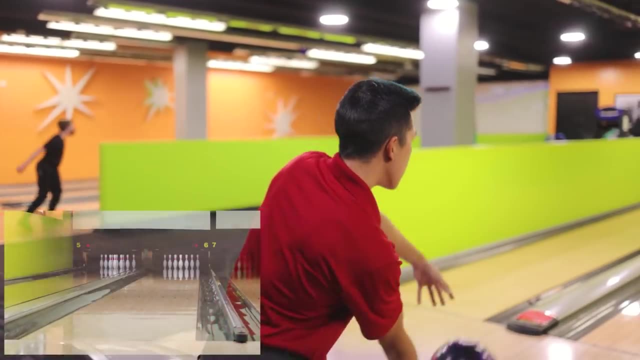 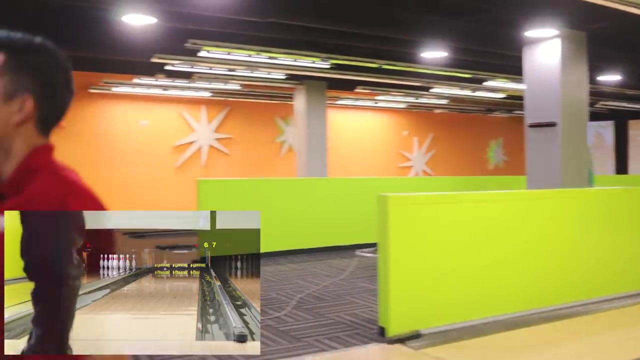 that I made with the pin down one. I'm just going to drop the speed Now. that shot I threw similar to the first shot with the pin down one, So let's see what the slower speed does for us. All right, It's kind of the same result, All right. So not quite what I expected, but this pin down one. 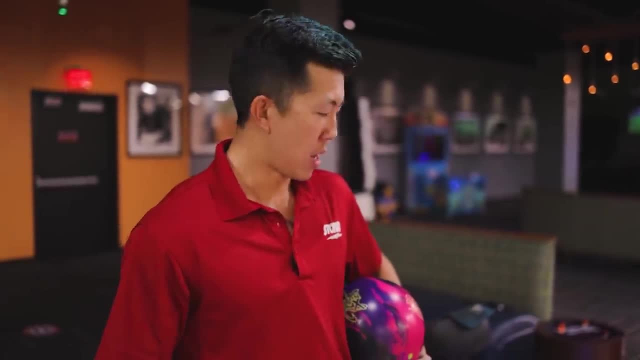 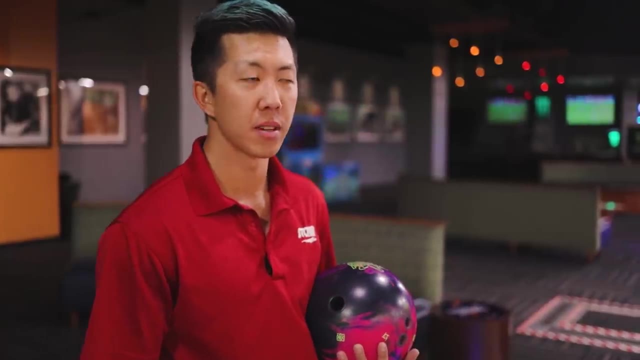 I've been throwing over there. I've literally thrown six times, So I think the cover is still fresh enough to bring the balls closer together. I've thrown the pin up one about 30 times, So not consistent really. We should probably get some more shots on the pin down one. 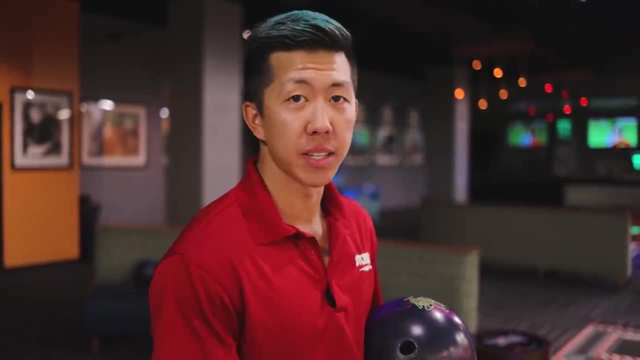 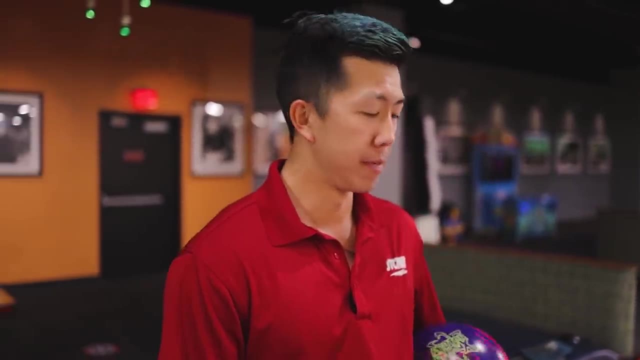 But considering how the distances down the lane look pretty similar, we can assume the pin down one will go longer. It's going to allow me to play straighter, And if I'm looking to hook the ball more, I'm going to go to the pin up one. We're going to move left just for the hell of it. 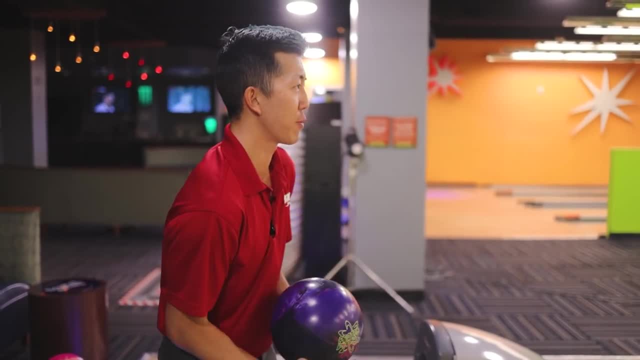 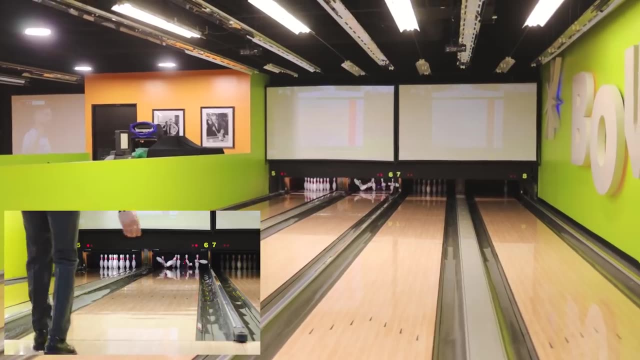 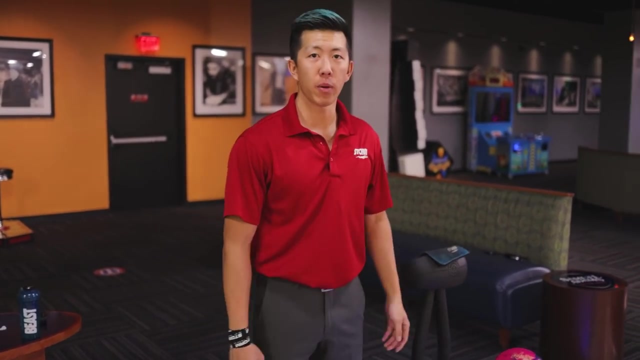 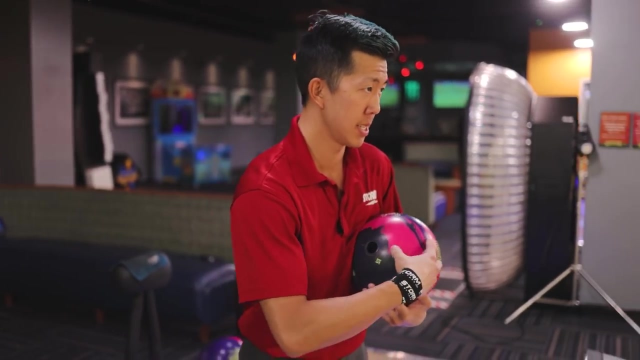 even though we're not quite flushing up the shots. Let's see if we can make it happen. That's actually pretty good, Pretty close. I kind of want to try that with the pin down one and see what happens. All right Back to the pin down one. I moved four with my feet and two with my eyes. 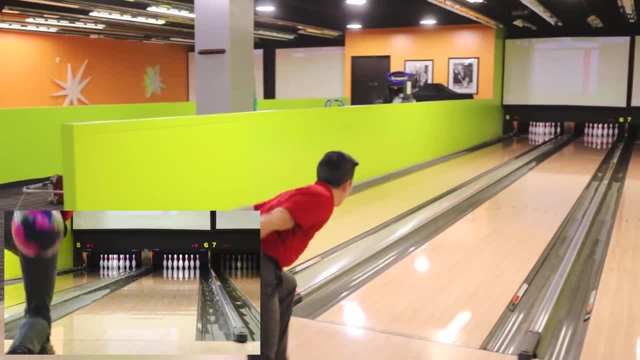 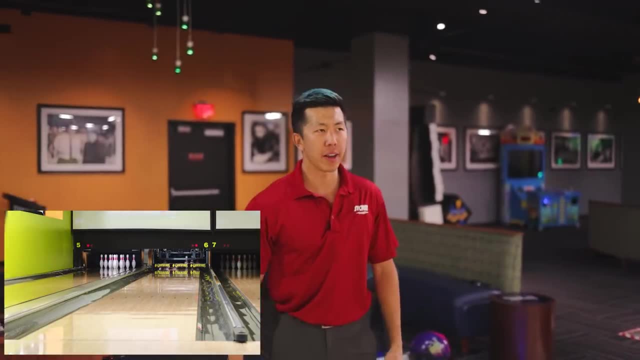 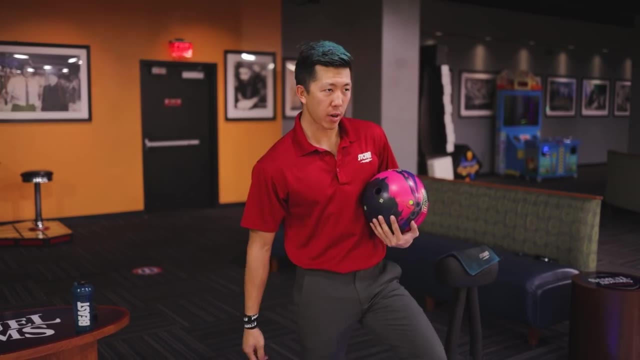 We're going to make the same shot here. Not in my best form right now. That was probably a good arrow left down lane. We'll give it another shot. All right, One more try. Same spot with the pin down. This one's a five-inch pin, like mentioned earlier. 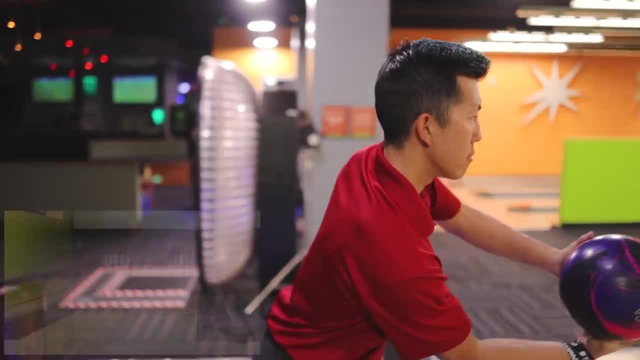 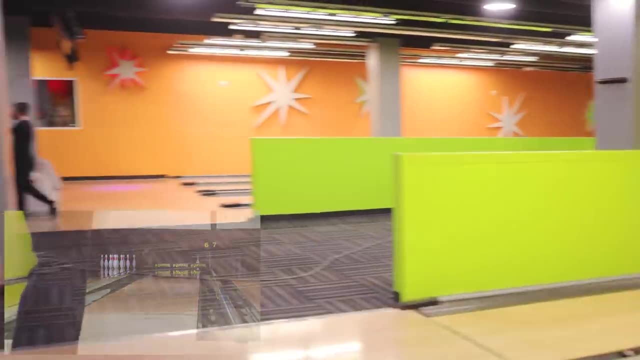 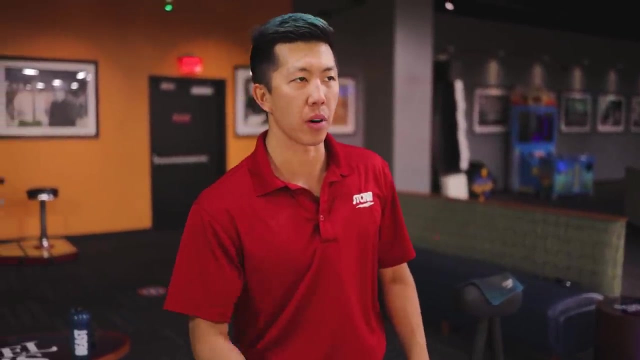 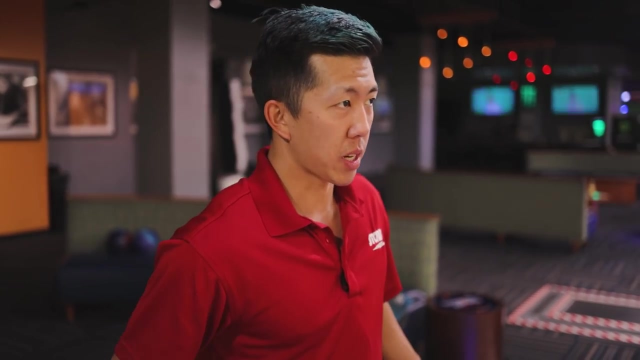 And let's see- All right, That was a little closer, Probably still a little further left than the pin up one, but you can visually see that ball kind of wobbling down lane And that's because the ball's not flaring as much And that's what's causing the ball to push further down the lane. All right, 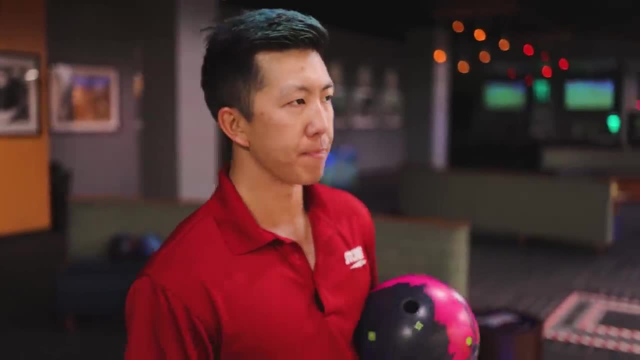 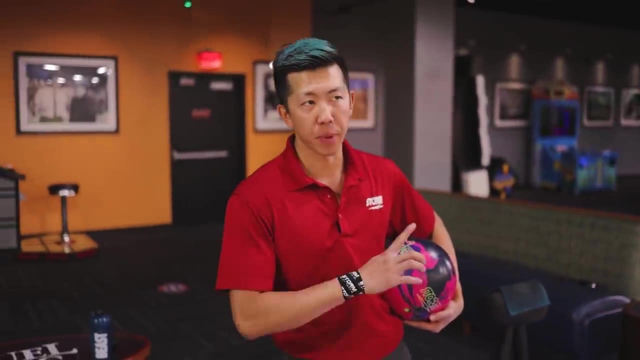 So, based off of that ring 10, I was manipulating it quite a bit, And you never really want to manipulate it when you don't have to. So with the pin up one it was a lot easier for me to shape the lane. This one I'm going to have to do a lot more to get it to go to the pin. 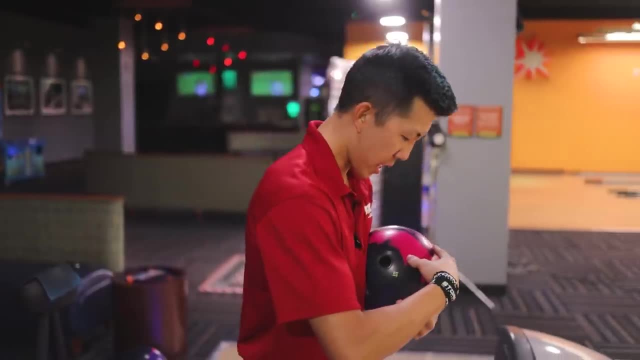 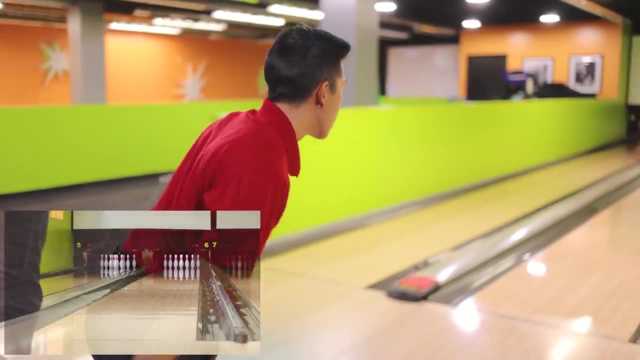 So I'm just going to move a few back to the right. Actually, I'm going to move even further right than where we started, just to see how we're looking in this part of the lane. All right, Cool. All right, All right.